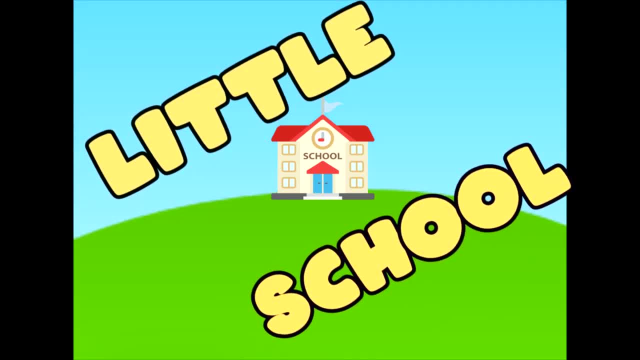 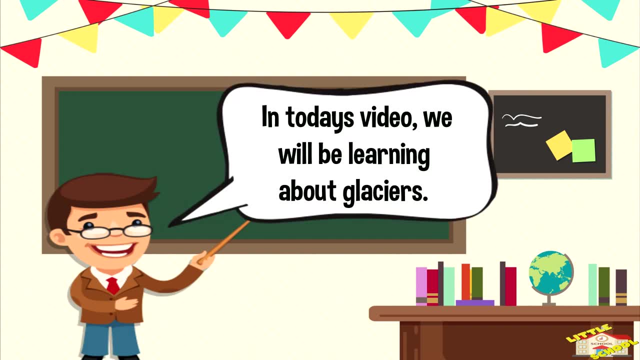 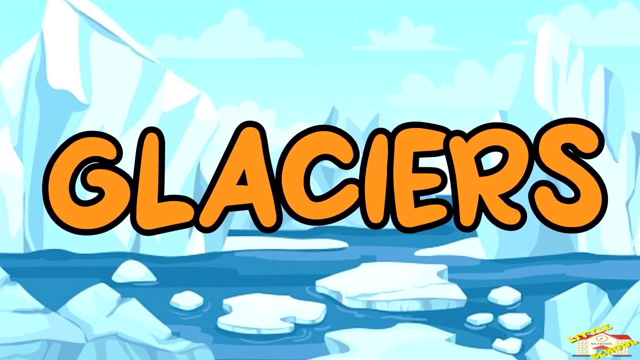 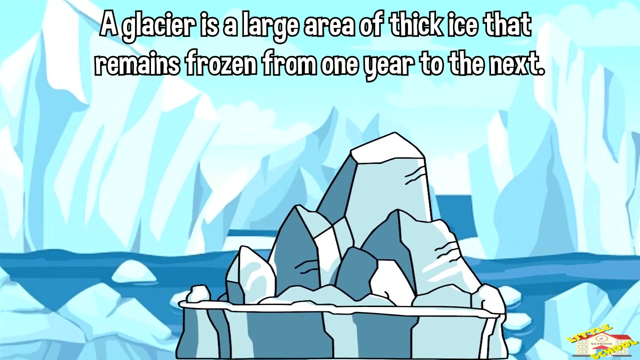 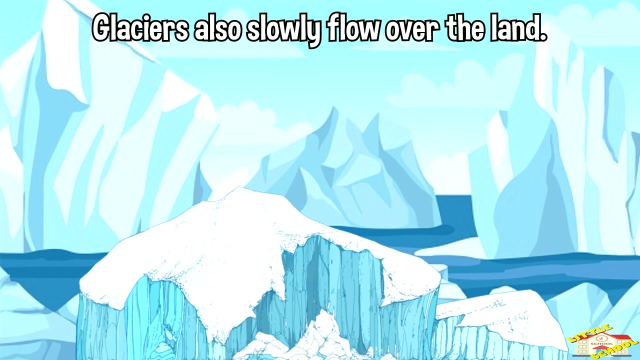 Hey kids, In today's video we will be learning about glaciers. Are you ready? Let's begin. A glacier is a large area of thick ice that remains frozen from one year to the next. Glaciers also slowly flow over the land. Thousands of years ago, large parts of the world were 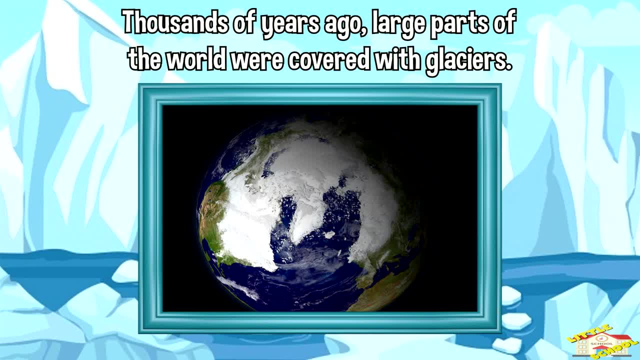 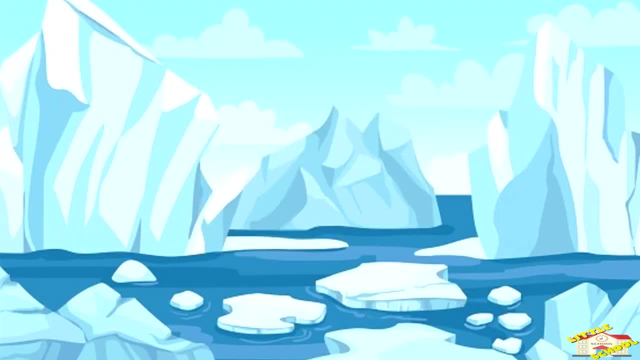 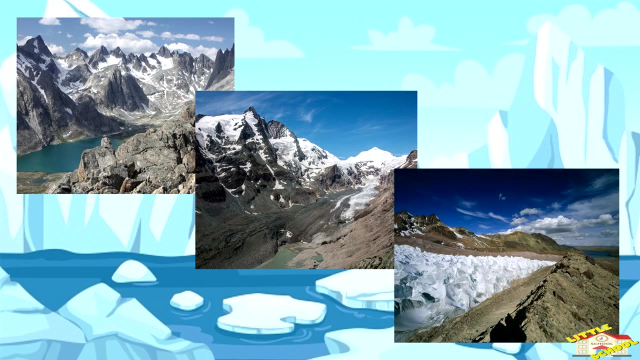 covered with glaciers. Glaciers exist all over the world. today, Most of Greenland is covered by thick sheets of glacier ice, as is Antarctica. There are small glaciers in the Rocky Mountains of North America, in the European Alps, in the Andes of South America. 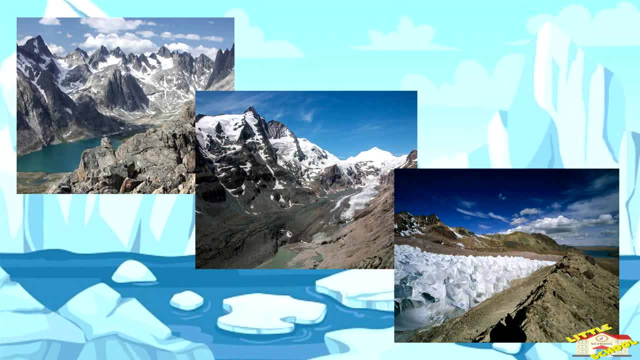 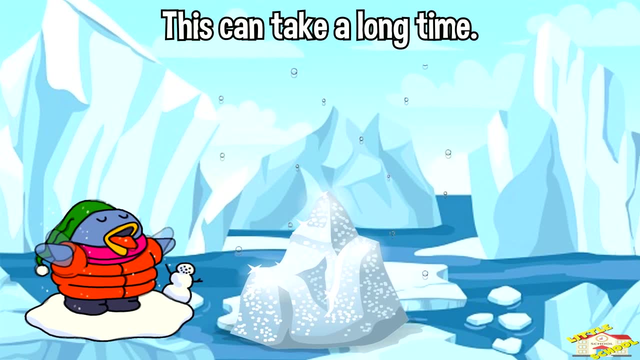 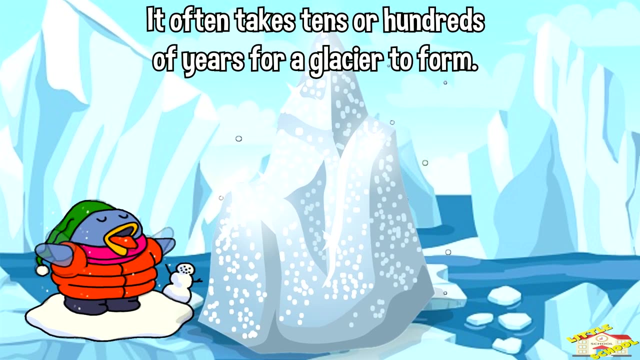 and even at mountainous points along the equator. Glaciers will only form in places that are cold enough and get enough snow. over time, This can take a long time. It often takes tens or hundreds of years for a glacier to form. There are two kinds of glaciers: continental. 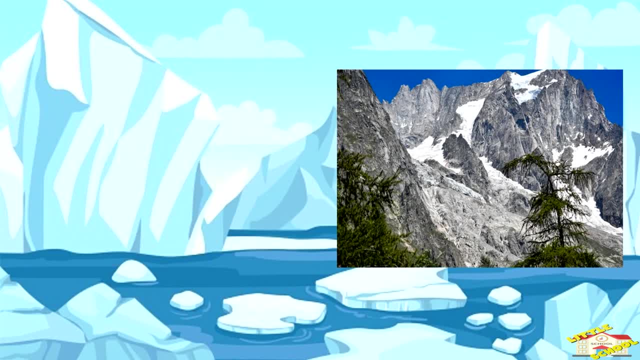 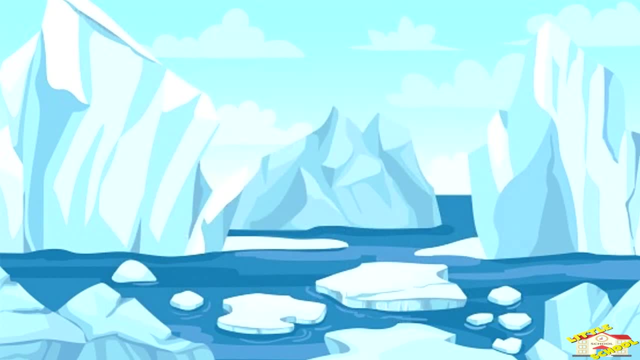 glaciers and mountain glaciers. Alpine glaciers are also called mountain glaciers. Continental glaciers are glaciers that spread out over a large area of land. They were created, mostly during the ice ages, a long time ago. There are still some continental glaciers in Greenland and Antarctica. 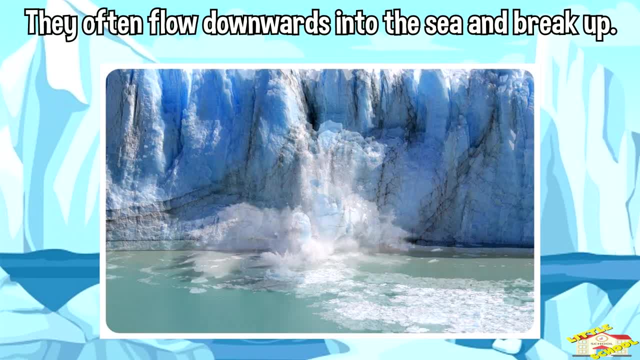 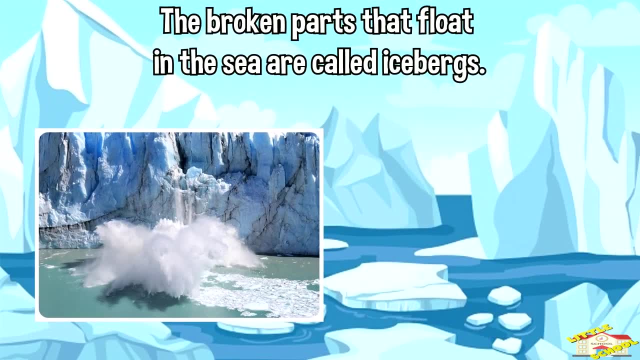 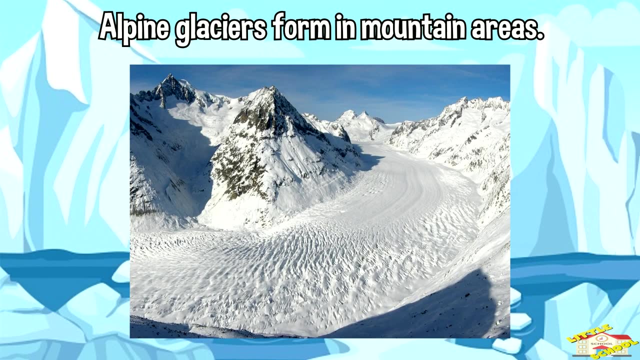 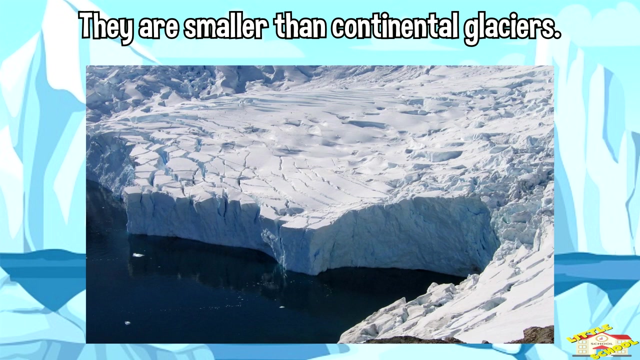 They often flow downwards into the sea and break up. The broken parts that float in the sea are called icebergs. Alpine glaciers form in mountain areas. They are smaller than continental glaciers. Alpine glaciers usually flow until they reach a point where they are completely.